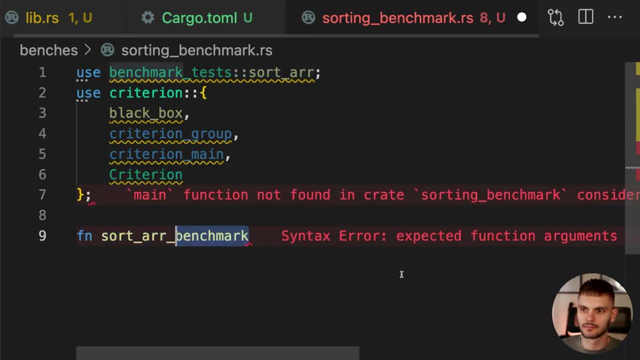 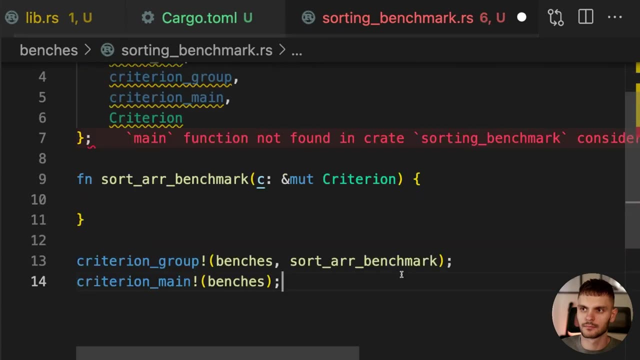 Next we'll set up our test function. The Criterion group macro is used to define a collection of functions to call with a common Criterion configuration. Next we'll set up our test function. The first argument is the name of the group, in this case benches, and the remaining arguments: 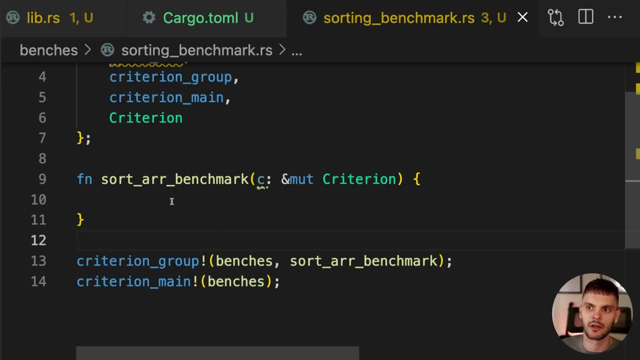 are names of functions. in this case we only have one function called sortArrayBenchmark And the Criterion main macro expands to a main function which runs all the benchmarks in a given group, in this case the benches group. With the setup complete, let's focus on our benchmark. 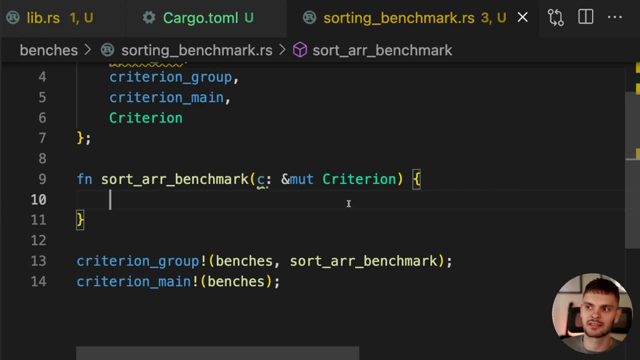 function. Each benchmark function gets access to an instance of the Criterion struct which allows us to configure and execute benchmarks. Each benchmark function gets access to an instance of the Criterion struct which allows us to configure and execute benchmarks. We'll use the Criterion struct to create a new benchmark, but first let's set up some data. 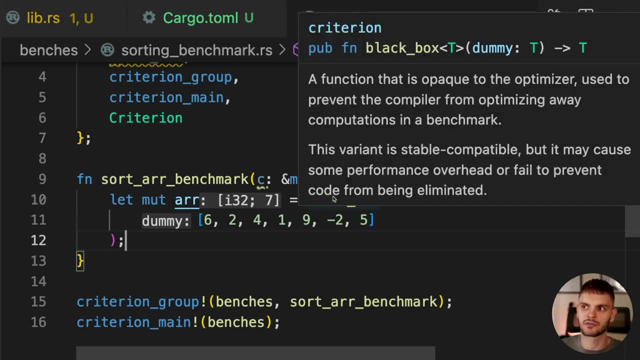 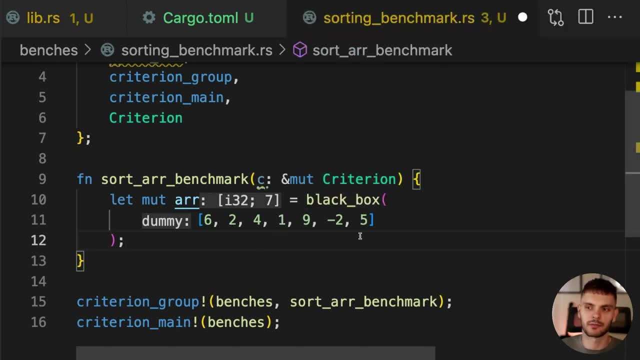 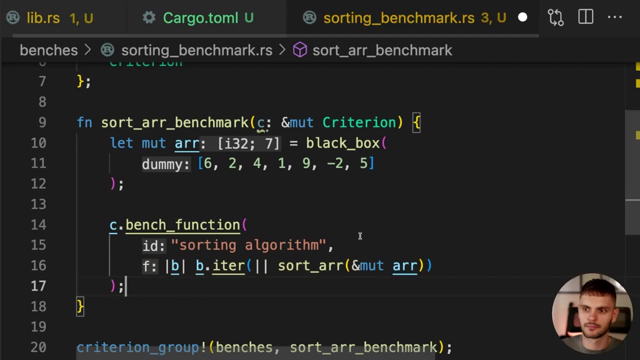 Here we created an unsorted array. we also use the blackbox function, which prevents the compiler from optimizing away computations in a benchmark. Next, let's create our benchmark. To create a new benchmark we call benchmark function on the Criterion struct instance. This function takes two arguments: an id and a closure. Inside the closure we get access to an. 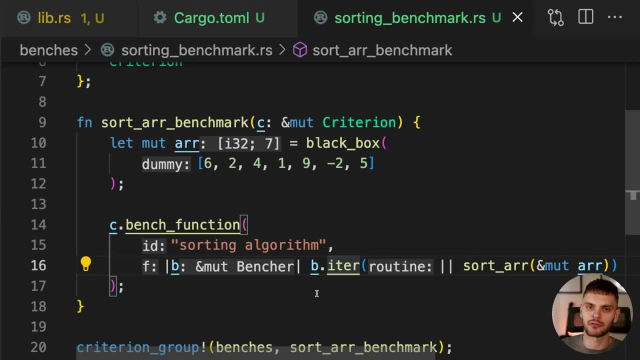 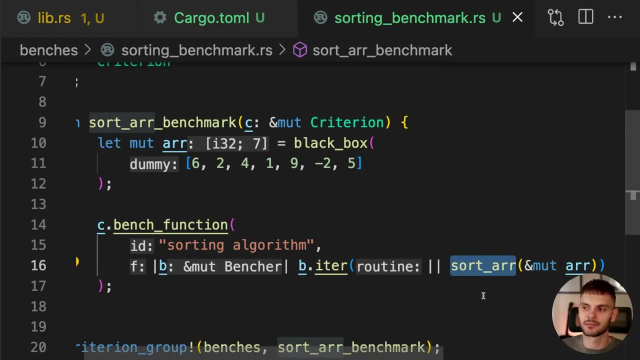 instance of bencher, which allows us to iterate a benchmark function to measure its performance. Inside the closure body we call the iter method, which takes another closure that executes our sort. The sort array function will be executed many times for its performance to be accurately measured, And with that our benchmark is now complete. Let's go ahead and run it. 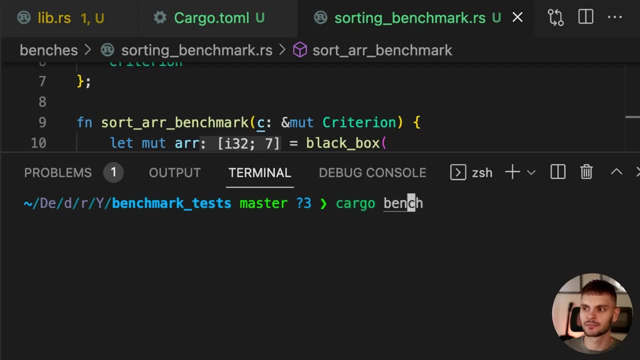 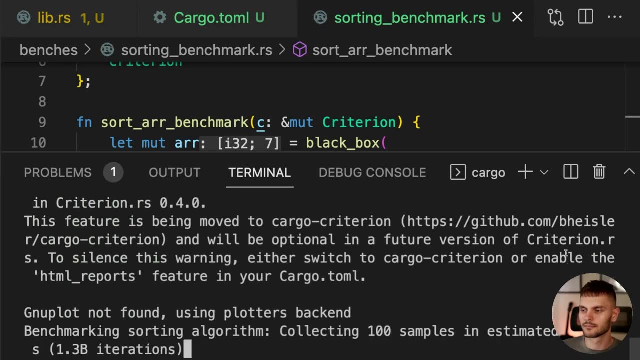 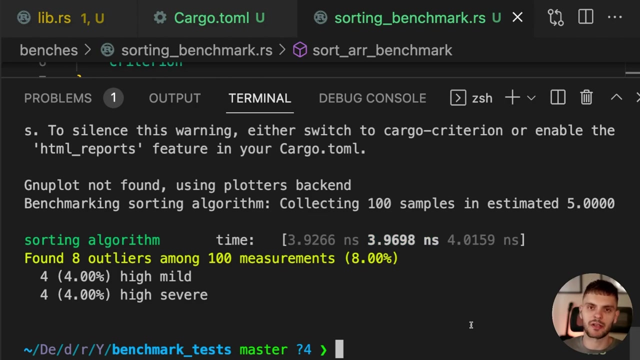 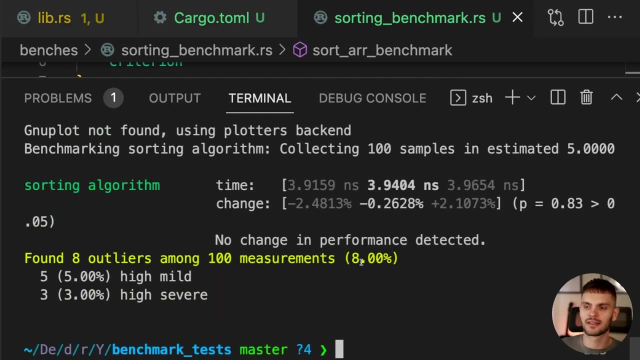 To run our benchmarks. we execute cargo bench. Our benchmark executed in about four nanoseconds. Let's run the benchmark again. This time we get a similar result and it even states that no change in performance was detected. Now let's go back to librs and change our sorting algorithm.